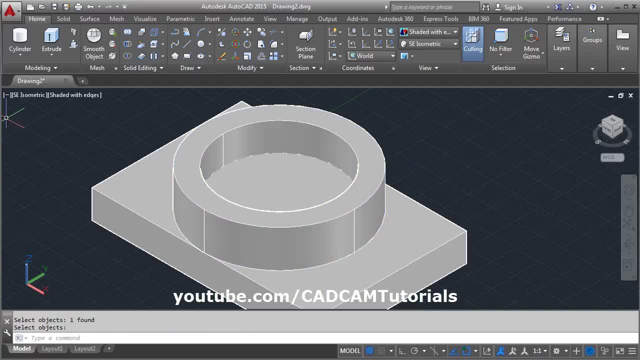 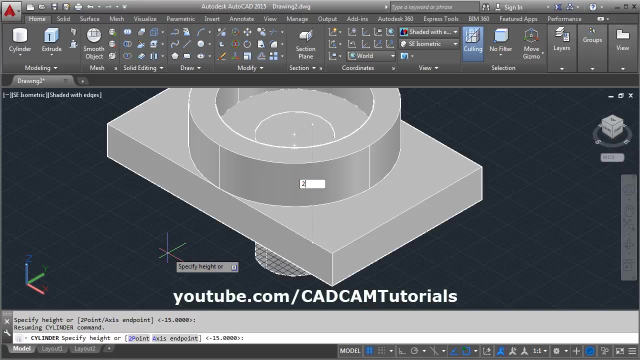 Select internal cylinder. Enter. Then next is this cylinder of dia 30.. Click on cylinder. Select center point. Give the radius of 15.. Enter. Give the depth of 20.. 20, because the difference between 20 and 15 is 5.. 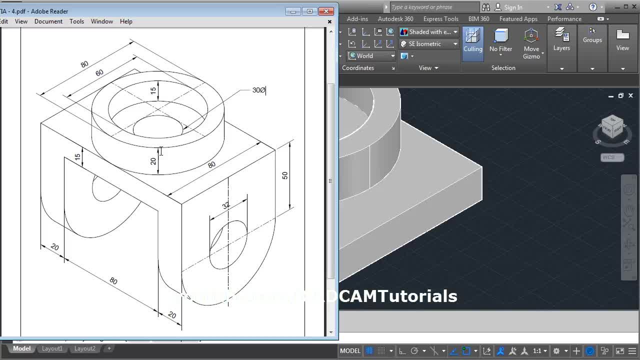 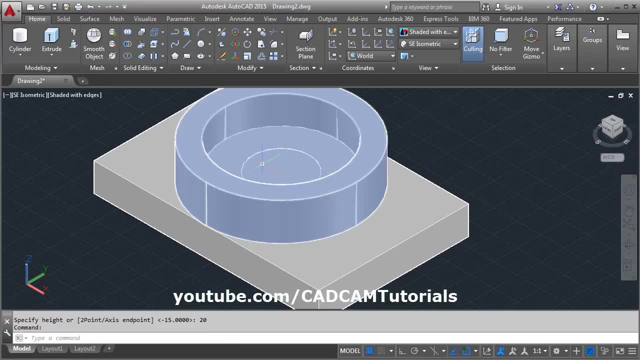 Here is 5 and here is 15.. Total depth will be 20.. Then give the direction below, Then give the depth of 20.. Again, we need a hole here. Click on subtract In this last link, select object to subtract this cylinder and this box. Then we need a hole for this cylinder. Click on subtract. Click on select object to subtract from this cylinder and this box. Click on subtract using this Répind object from this cylinder. In this next link we will see some groin. Click on subtract object from this cylinder. 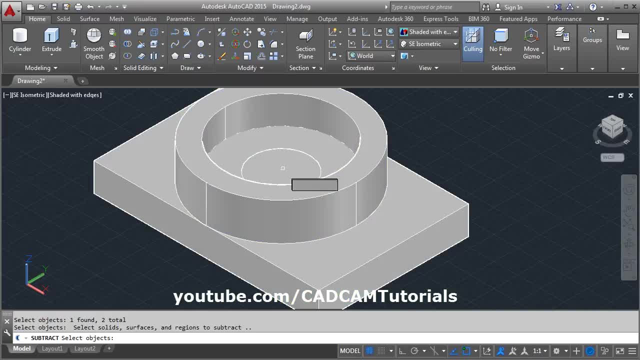 Then click on subtract or in this next name we will have the total depth. Then click пожалуйста down. Click on subtract. The next item are moving super specific. Click on subtract the object from this cylinder, enter. then select this internal cylinder, enter. it has subtract properly. then next. 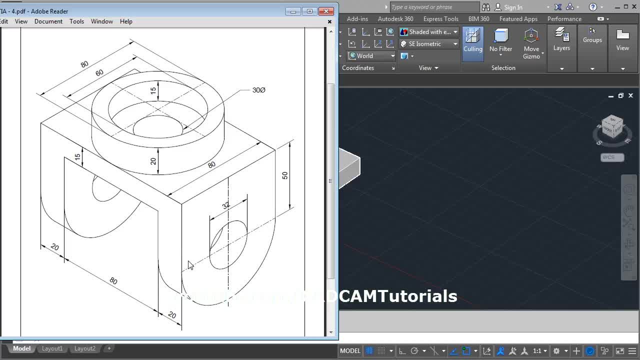 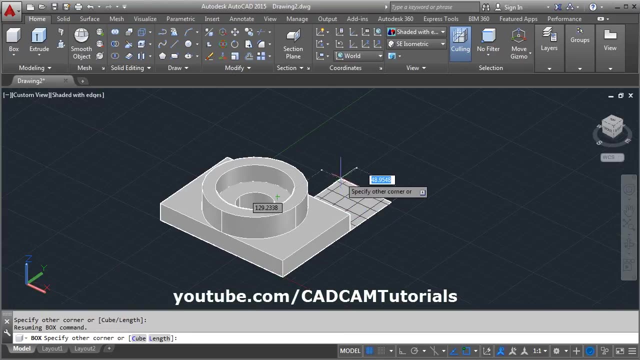 will be to create this box of 20 width, 80 length and 50 or 35. we will minus this 15 from this 50. that is certified depth. take the box command, give the first point, take it inside, give the width of 20, tab length of 80, enter and. 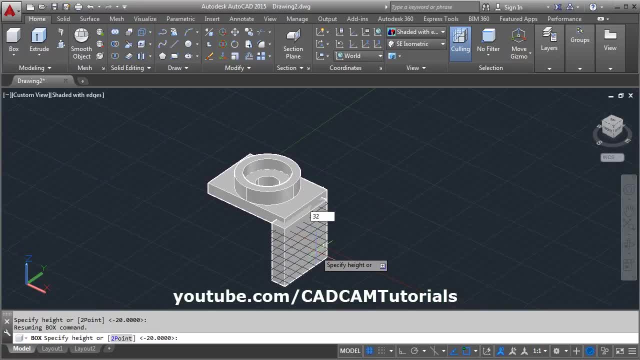 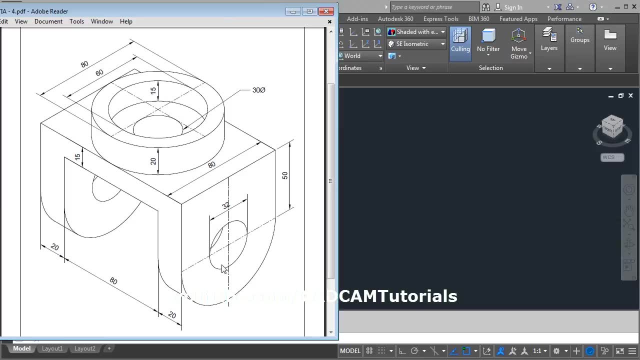 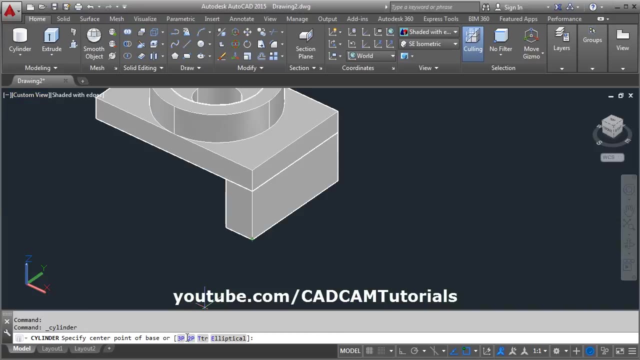 take cursor down, give the height of 35, enter, make the grid off. then next will be this cylinder: click on cylinder. click on this two point option. take the this first point, take the second point. then we need it. vertical click on this axis endpoint, make ortho on and horizontal axis in this direction and 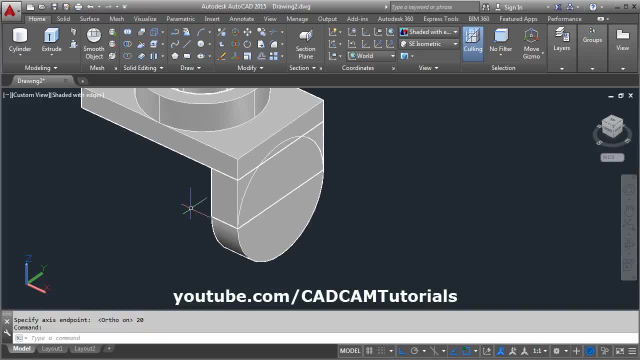 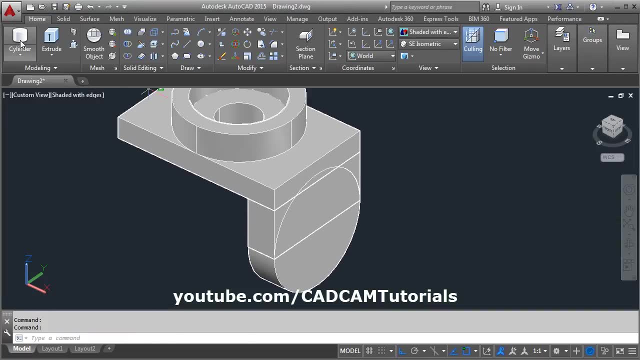 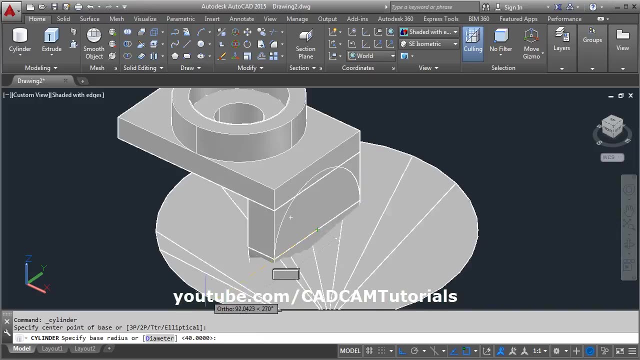 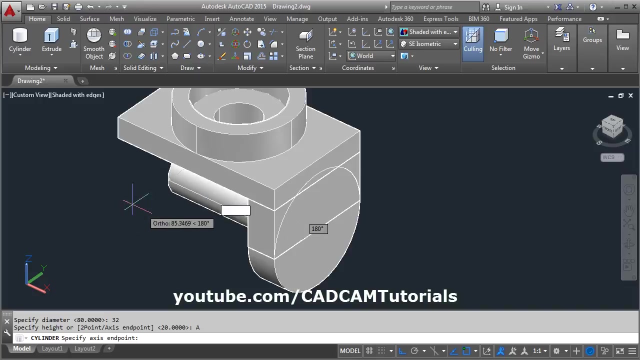 depth is 20, enter. then next will be internal cylinder of 32 diameter. click on cylinder, give the center point and then give diameter of 32, мам of 32, then give the axis end, take it inside and give the depth of 20, then we.